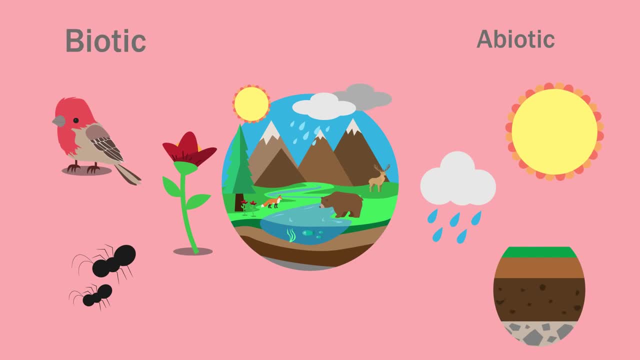 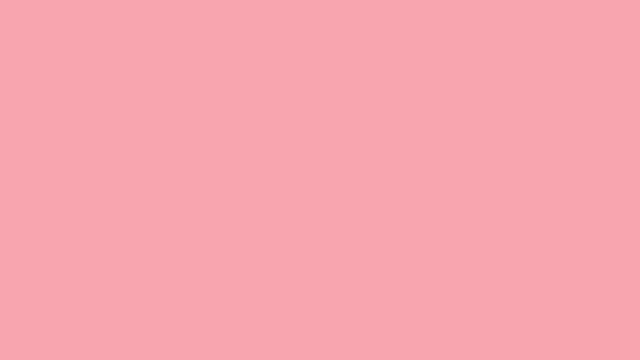 components. ecosystems are composed of both biotic or living, and abiotic or non-living components. Let's start by discussing the abiotic parts of an ecosystem. Sunlight, precipitation, soil composition, temperature and air currents are all examples of abiotic components that can 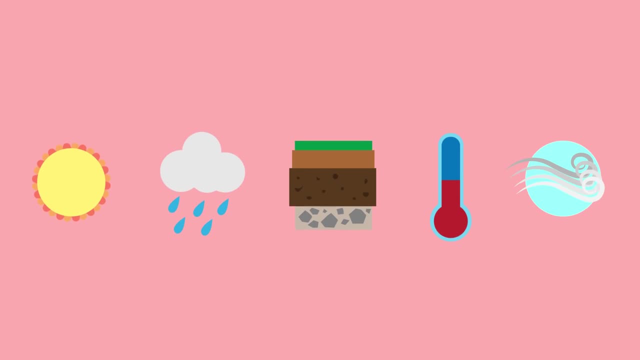 be found within an ecosystem. While each of these components is important by itself, how they interact with each other also greatly influences their environment. For instance, in places like tropical rainforests, precipitation almost always comes in the form of rain because of the high 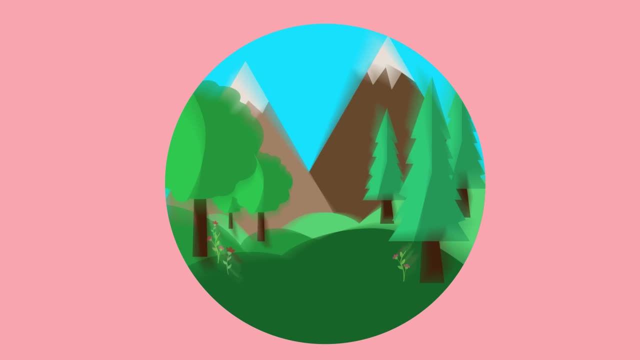 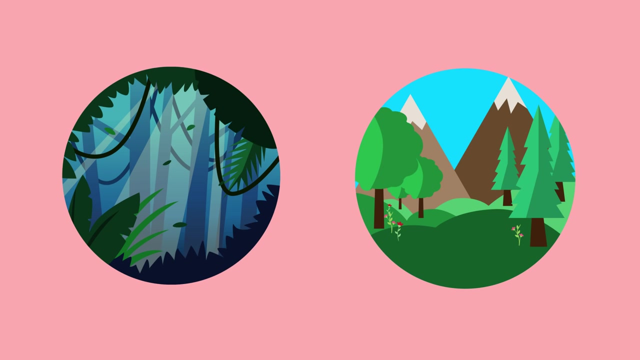 average temperature. However, in places like temperate forests, where temperatures are much more variable, a much wider variety of precipitation types exist. Even though the two habitats are both dominated by trees, the difference in temperature ranges results in vastly different precipitation types and amounts. The variation in temperature and precipitation also affects the local wildlife. 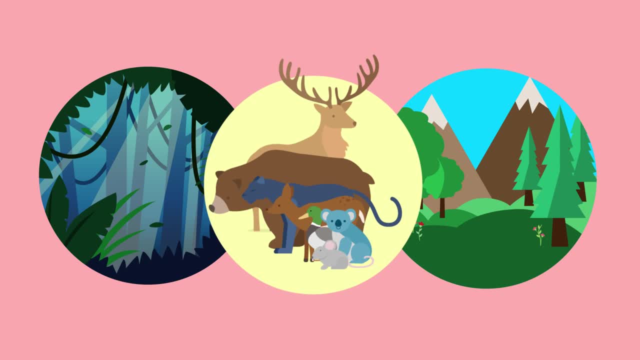 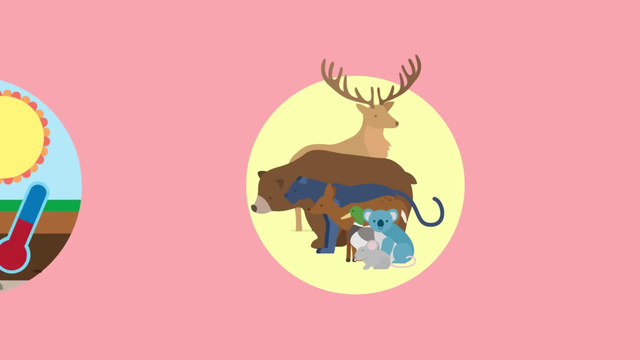 a biotic component and helps determine which species can survive in a given ecosystem. The biotic components of an ecosystem also interact with one another, much like the abiotic components. One of the best examples of this is how the various trophic levels interact. 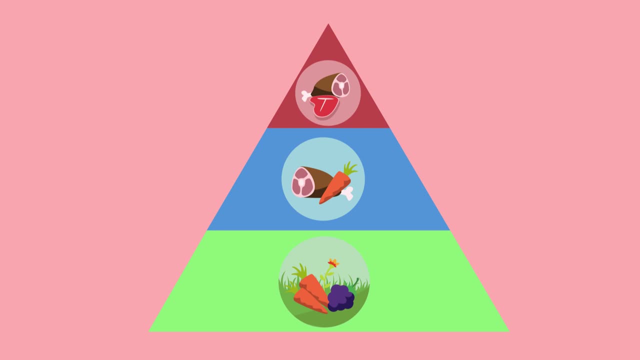 with each other. A trophic level is how scientists classify animals based on their food preferences. At the lowest trophic level are the herbivores, those animals that primarily eat plants. In the next highest trophic level are the animals that eat the herbivores, as well as some plants known as omnivores. 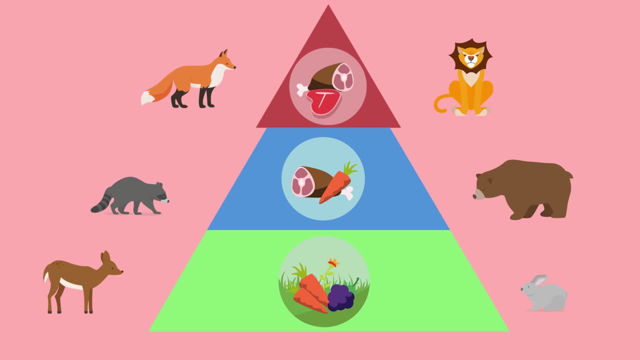 The highest trophic level is the carnivore and is represented by animals such as wolves, lions and eagles. Each of these trophic levels interacts with the other either directly or indirectly. A direct interaction between trophic levels usually takes the form of one organism consuming another. 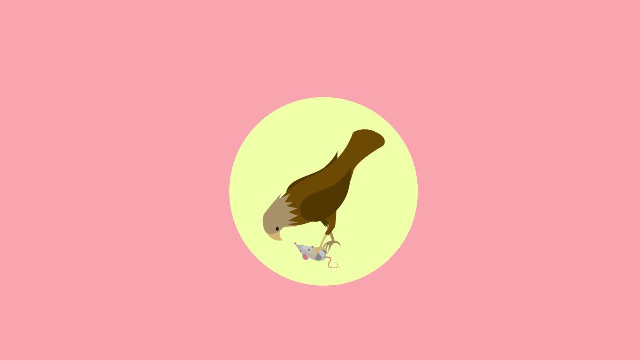 such as when hawks eat mice. An indirect interaction can be a bit harder to see, but often occurs when there is an intermediate step involved between two trophic levels interacting. Using the previous example, berries frequently consumed by mice are able to grow better as a